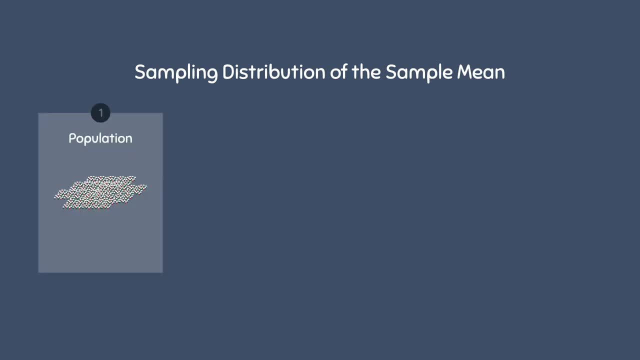 of the sample mean. the first step is to find your population of interest. Let's say we were interested in measuring height. Next you would take a random sample of size n. Now we'll measure the heights of each individual in this sample. Once that's complete, we 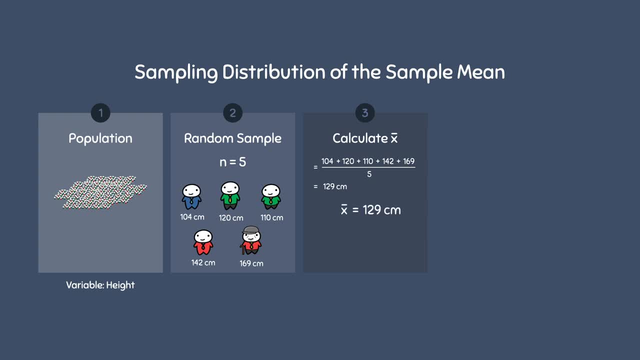 will calculate the mean height, x-bar for that sample And then, finally, we would create a frequency distribution of the sample mean by plotting the value of x-bar for this sample. Remember that a sampling distribution involves taking multiple samples, so we would have to do this entire process for another sample. Therefore, we would take another simple, random. 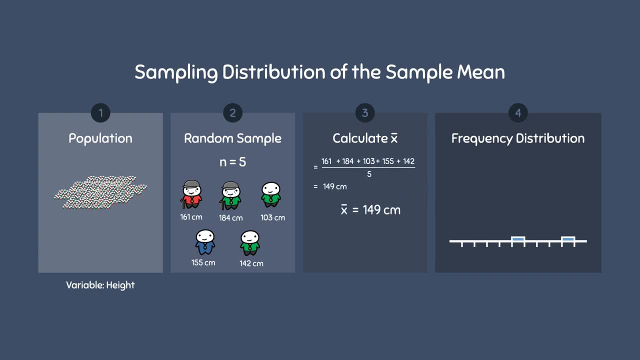 sample, calculate x-bar and then plot that value onto the histogram. Take another random sample, calculate x-bar and then plot that onto the histogram. If we repeatedly do this hundreds and thousands of times, we eventually end up with a sampling distribution. Essentially, a sampling distribution is just a whole bunch of x-bars that are stacked. 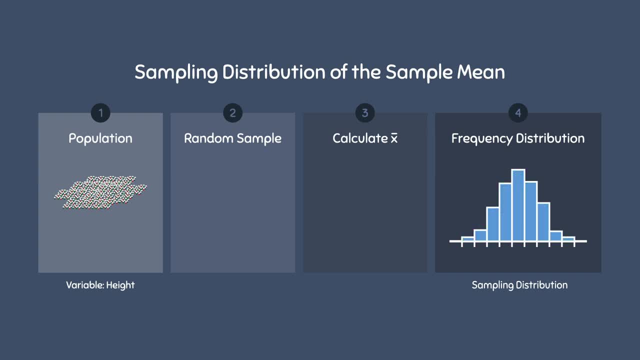 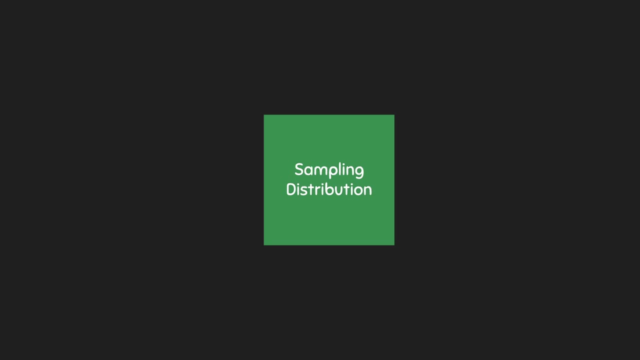 on top of each other. And the interesting part is, if you have enough data, the sampling distribution will be normally distributed. This is due to the central limit theorem, but we will save the discussion for this topic in the next video. So now that you know what a sampling distribution is, let's compare the difference between: 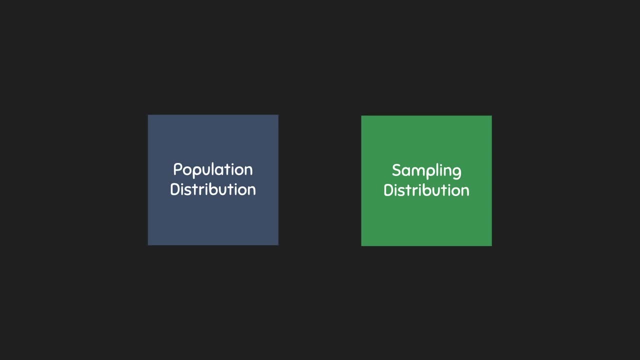 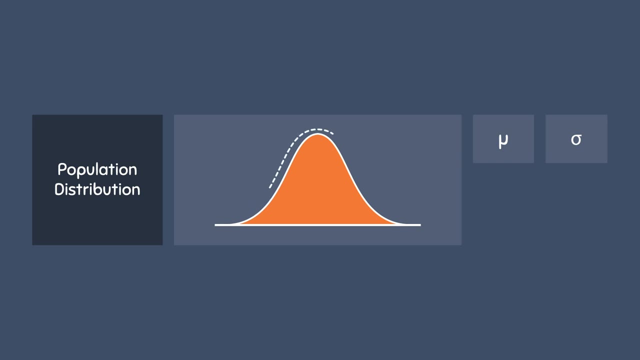 a population distribution and a sampling distribution. A population distribution has a mean of mu and a standard deviation of sigma, And when a random variable x follows a normal distribution with a mean mu and a standard deviation sigma, this can be represented by the following notation And the standardization formula for this: normally, 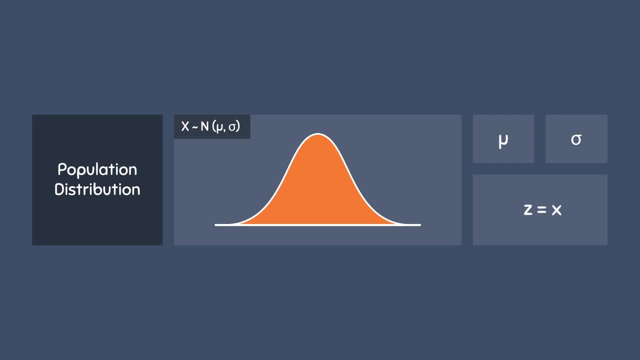 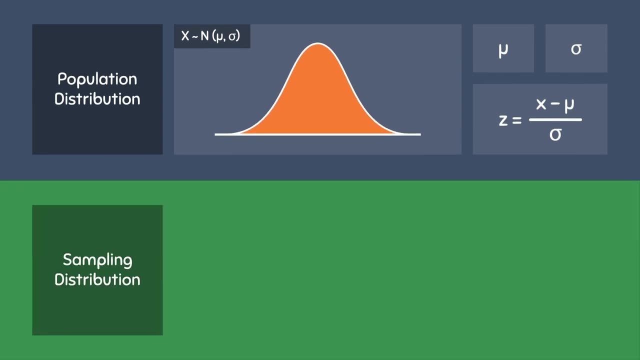 distributed population would be equal to an observation x minus the population mean mu divided by the population standard deviation sigma For the sampling distribution. this is created by taking multiple random samples from the original population, then calculating the x-bar for each sample and then combining 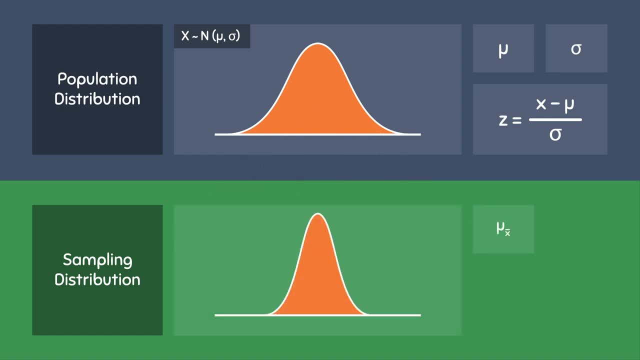 it into one graph. When we do this, we find that the population mean of all the x-bars is actually equal to mu. In other words, the mean of the sampling distribution is equal to the mean of the original population distribution that you sampled from. However, for the standard, 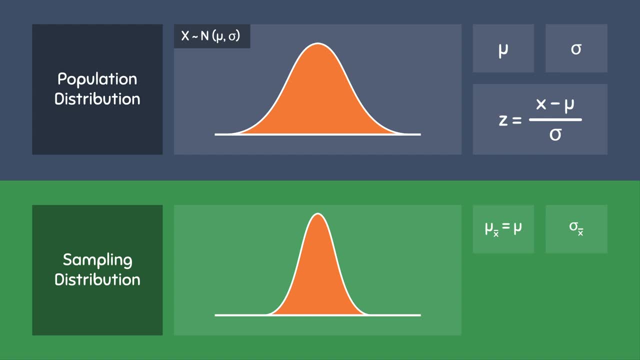 deviation. there is a응 mu and we can clearly see that we have something different between these two graphs. The sampling distribution has a much smaller spread than the population distribution, which clearly has a larger spread or a larger standard deviation. The standard deviation for a sampling: 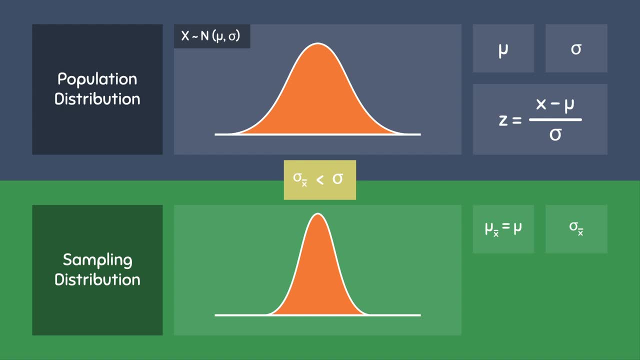 distribution is always smaller than the population standard deviation. This is because the averages are less variable than individual observations, and we know that a sampling distribution is made up of averages, whereas a population distribution is made up of individual observations. wide range of measurements and therefore more variability. 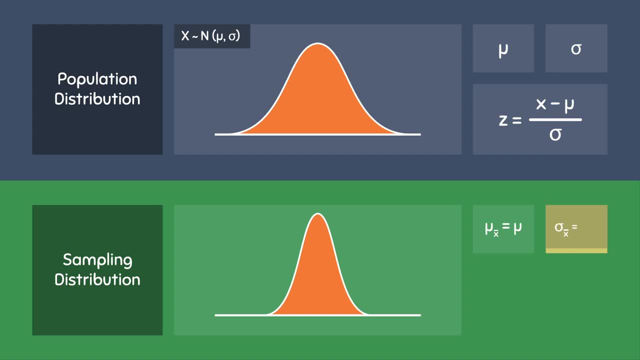 We find that the standard deviation for a sampling distribution is equal to the population standard deviation sigma divided by the square root of n, where n is the size of your sample. The standard deviation of a sampling distribution is also called the standard error. So when a random variable x follows a normal distribution with a mean mu and a standard, 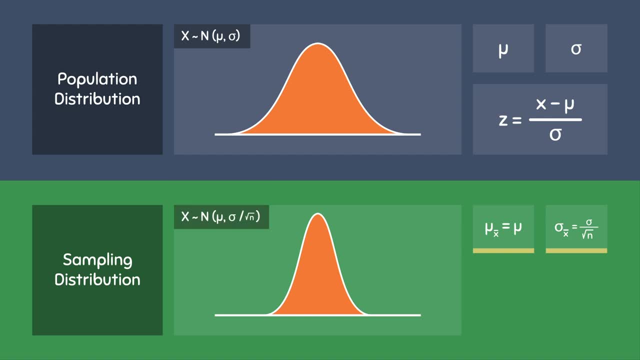 deviation of sigma over the square root of n. we can write this as a notation to formally state that: And finally, the standardization formula for a sampling distribution is equal to an observation: x minus the population mean mu of all the x bars, which is just equal to mu divided. 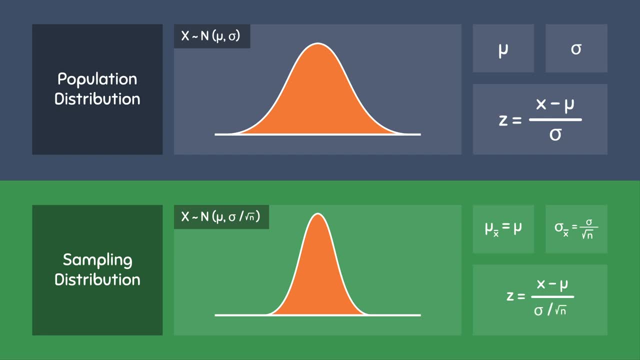 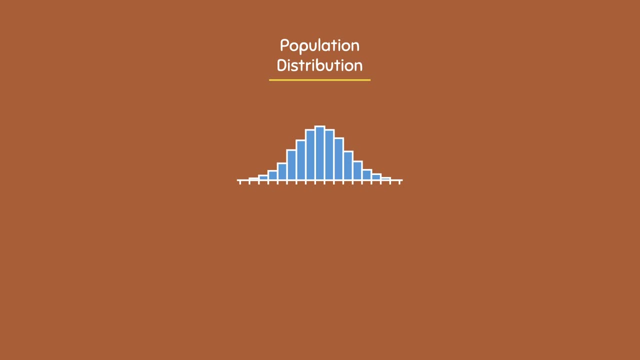 by the standard deviation, which is equal to sigma divided by the square root of n. So to quickly recap what we've talked about, a population distribution is a distribution that is created for measuring every single individual in the population. A sample distribution is a distribution that 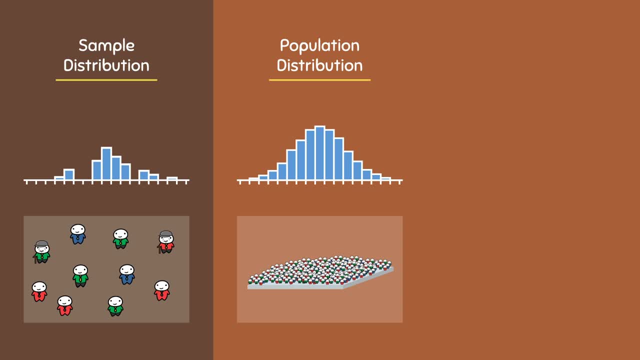 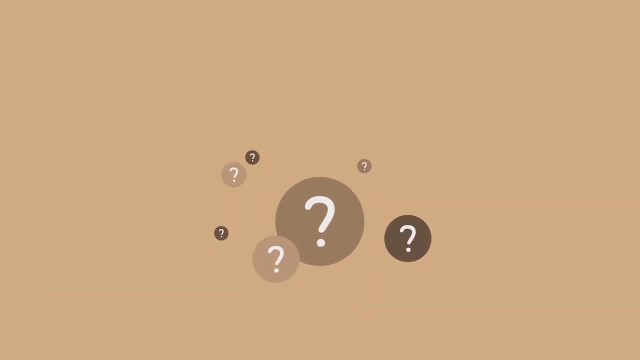 is created for measuring every single individual in the sample And, most importantly, a sampling distribution involves repeatedly taking a sample and calculating a statistic for each individual sample and then combining that information to create a distribution. Now you might be asking what's the point of a sampling distribution in the first place? 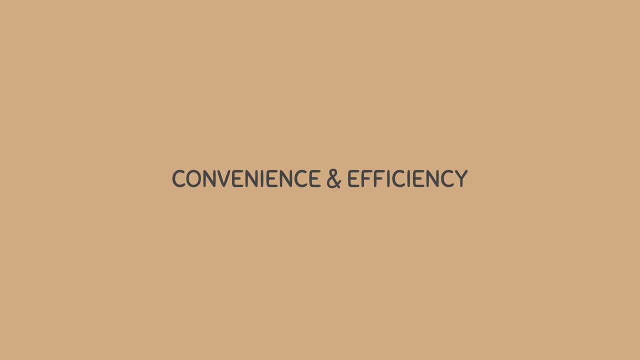 And to answer that question, it all boils down to convenience and efficiency. For example, if we wanted to know the average height of all humans living on earth, we would first have to measure and record the heights of every person on earth. As of 2021, there are about 8 billion people living on earth right now. 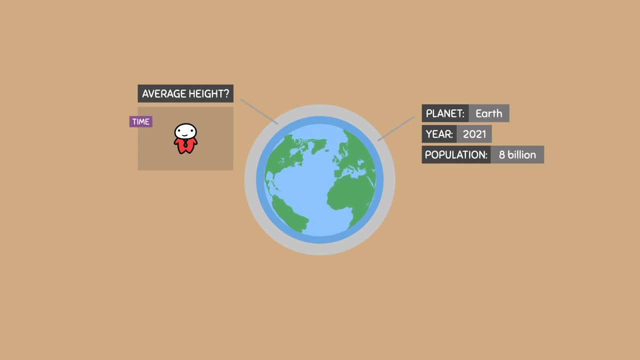 That's a lot of people. Measuring every single person would take a lot of time, effort and money. So instead we can create a sampling distribution And from this sampling distribution it can give us an idea of what the value of the population. 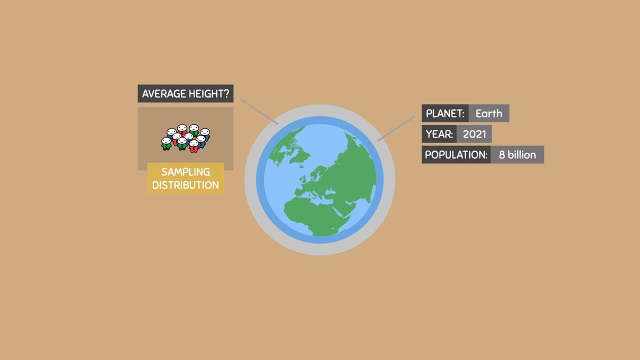 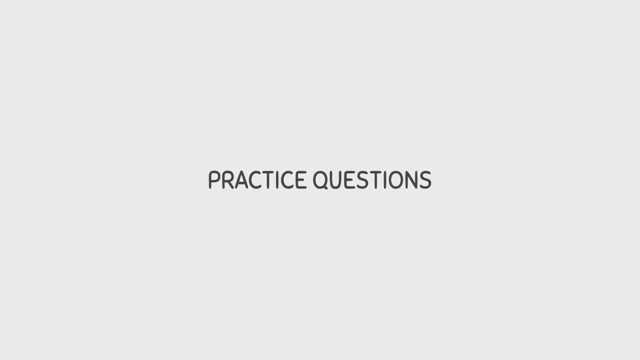 mean mu is, without having to measure every single individual on earth. Another great thing about the sampling distribution is that it allows us to calculate the probability of getting a certain outcome based on what our sample size n is equal to. So now that you know what a sampling distribution is, let's do some practice questions. 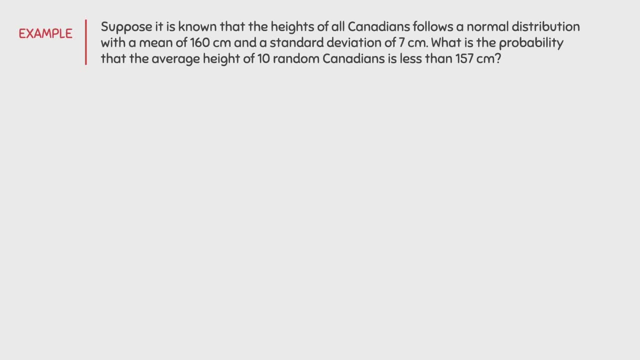 Suppose it is known that the heights of all Canadians follows a normal distribution, with a mean of 160cm and a standard deviation of 7cm. What is the probability that the average height of 10 random Canadians is less than 157cm? Before I solve this question, I'm going to make some illustrations to help you understand. 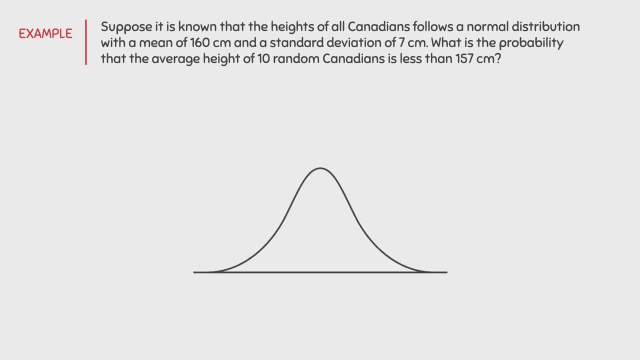 what is happening? According to the question, we have a normal distribution with a mu of 160 and a sigma of 7.. Mu is always located in the center of the distribution, so we will put 160 in the center. From here we can create intervals that increase by the standard deviation. 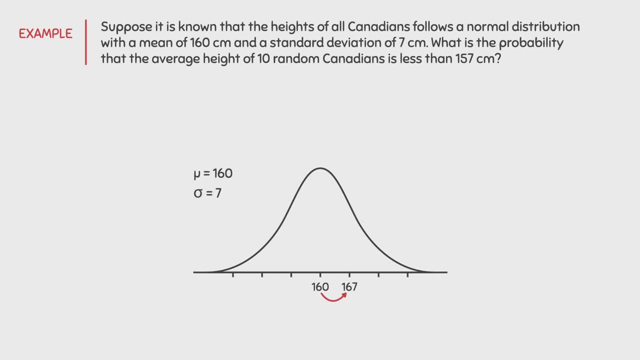 So one standard deviation to the right of the mean is 167,, two standard deviations to the right of the mean is 174, and one standard deviation to the left of the mean is 153, and so on and so forth. This is the population distribution. 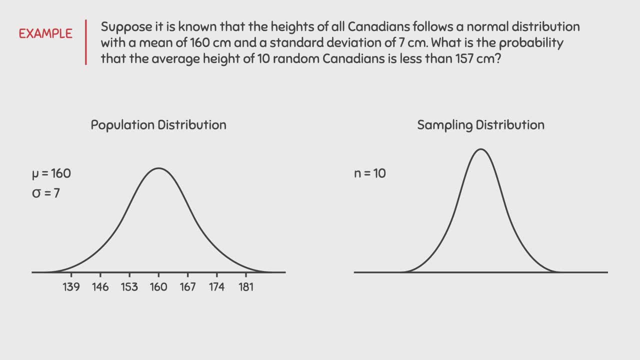 For the sampling distribution of the sample mean. we know that n is equal to 10, because the question says that this is the size of the sample we are dealing with. We also know that mu x bar is always equal to the mean of the parent population. so it 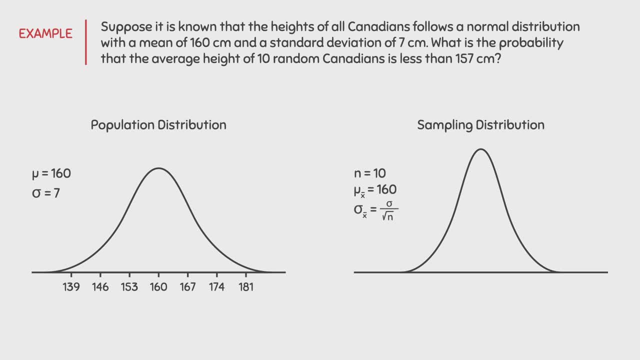 will also be equal to 160cm. However, the standard deviation of the sampling distribution is equal to sigma divided by the square root of n. In this case, the standard error is equal to 7 divided by the square root of 10, giving: 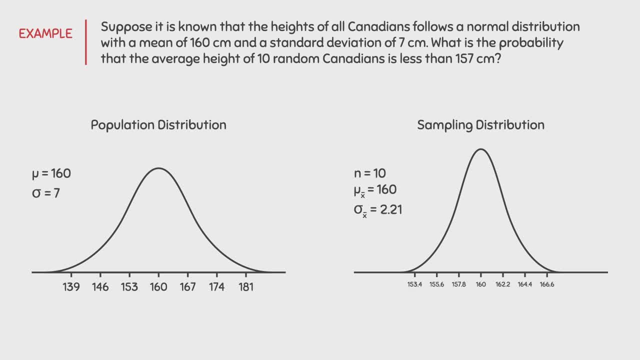 us an answer of 2.21.. This means we can create intervals that increase by the standard deviation. Now that you can visually see the difference between the population distribution and the sampling distribution, let's tackle the question: What is the probability that the average height of 10 random Canadians is less than 157cm? 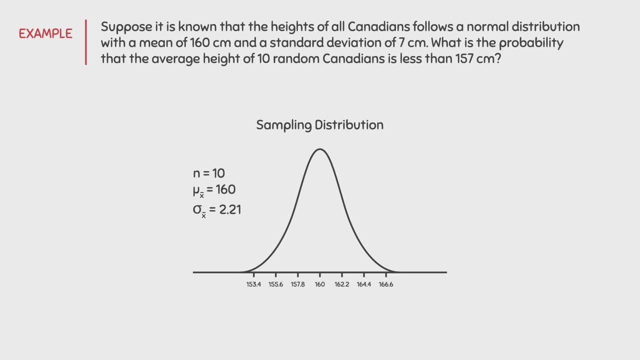 This refers to the sampling distribution, not the population distribution. Therefore, this is the area we are concerned about. We are looking for the proportion of x less than 157. And this is unknown until we standardize the distribution. so we will use the standardization. 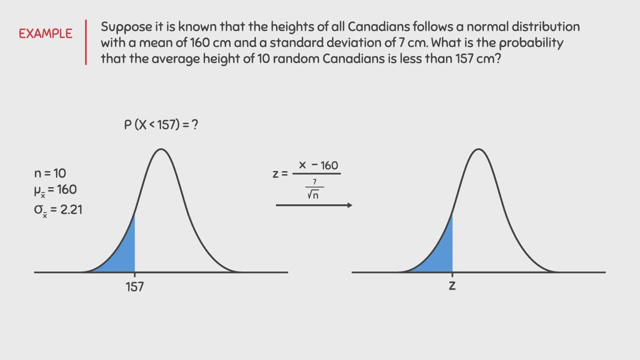 formula: Mu is equal to 160, sigma is equal to 7, and n is equal to 10.. We can replace the entire denominator by the standard error, which we have already calculated to be 2.21.. All we have to do now is plug 157 into the formula, and when we do, we get a z-score. 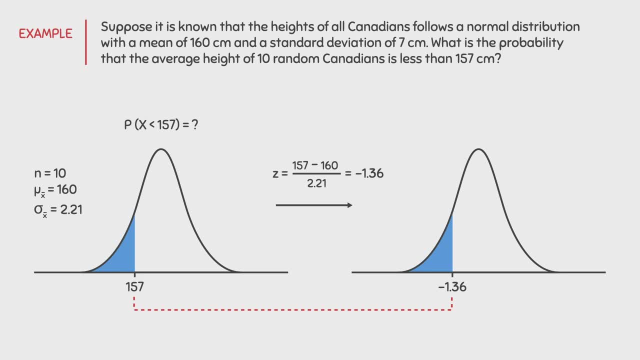 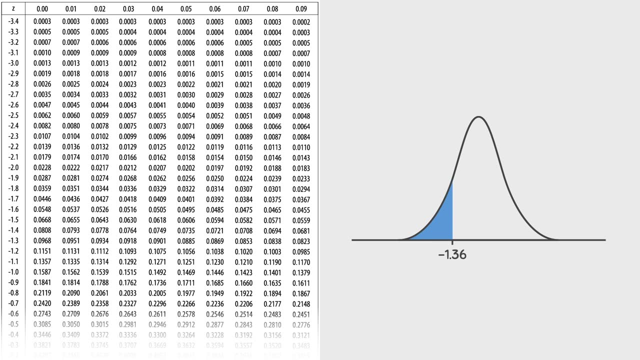 of negative 1.36,, which corresponds to our x-value of 157.. Now we can use the z-score table to calculate the standard deviation. Let's do it together to determine how much area is associated with this z-score According to the table. 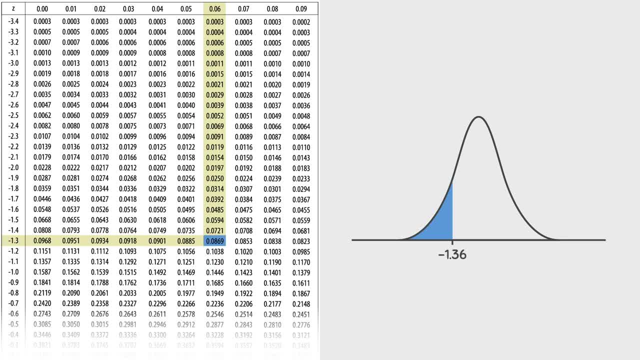 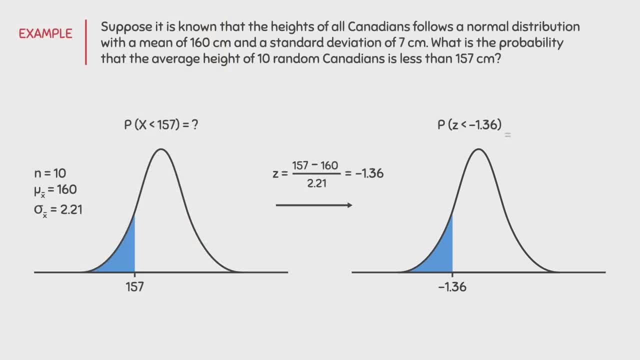 a z-score of negative 1.36 corresponds to an area of 0.0869.. Therefore, we can say that the proportion of z less than negative 1.36 is equal to 0.0869.. This value is, in fact, the same proportion. 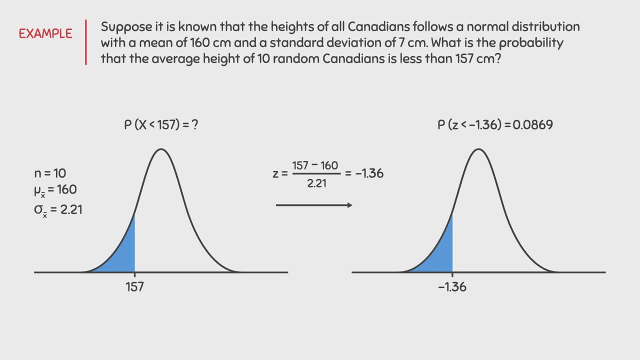 of x less than 157.. As a result, we can say that the probability that the average height of 10 random Canadians being less than 157 is equal to 0.0869 or 8.69%, and that is the answer. 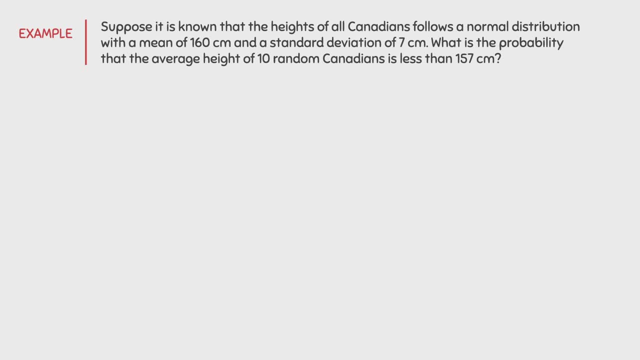 For the next example, I'll introduce a part 2 to this question. What is the proportion of all people that have heights greater than 170 cm? For this question, it's important you understand that we will not be dealing with a sampling distribution anymore, and this is because the question asks for all people. Therefore, 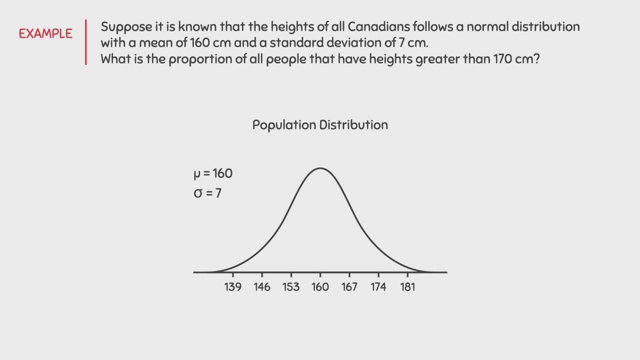 we are going to be working with a population distribution. instead, We are looking for the proportion of x greater than 170.. In order to find this area, we need to standardize the distribution, and we will do this by using the standardization formula. 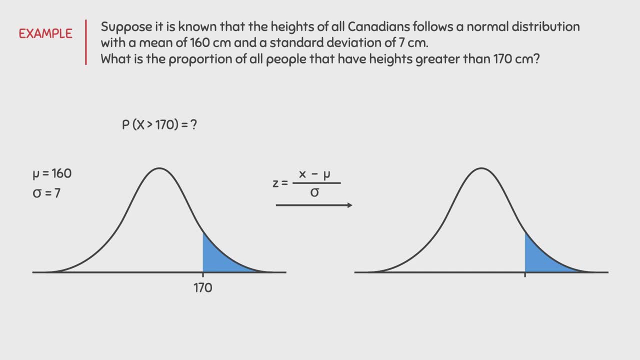 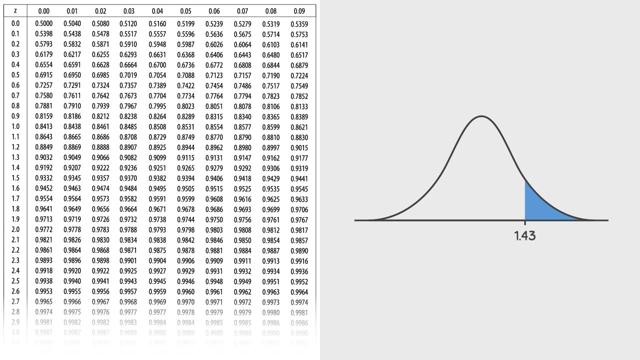 This time we have to use the formula for the population distribution rather than the formula for the sampling distribution. Plugging 170 and everything else into this formula gives us a z-score value of 1.43.. From here we can use the z-score table to see how much area is associated with this z-score. A z-score value of 1.43 and the total in the form of 0.8 is the sum of all the values of the number higher than 170.. We want to have only the z-score value, which is distributed by the formula. 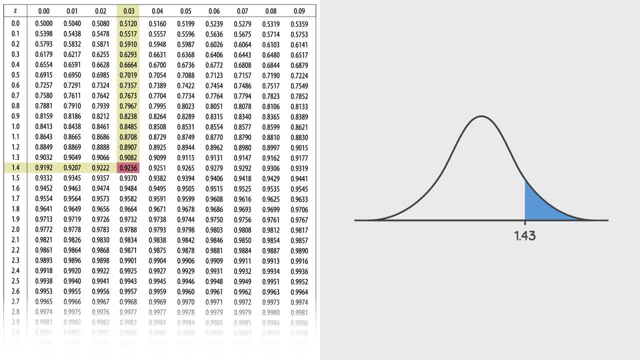 of 1.43 is associated with an area of 0.9236.. However, remember that the z-score table only gives us areas to the left of a z-score value. According to the table, a z-score of 1.43.